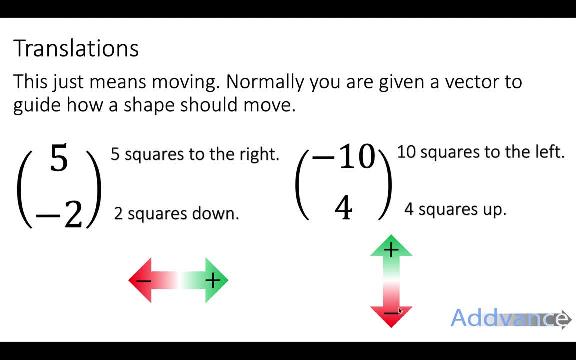 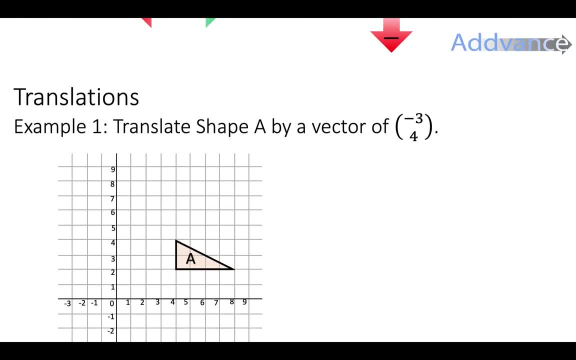 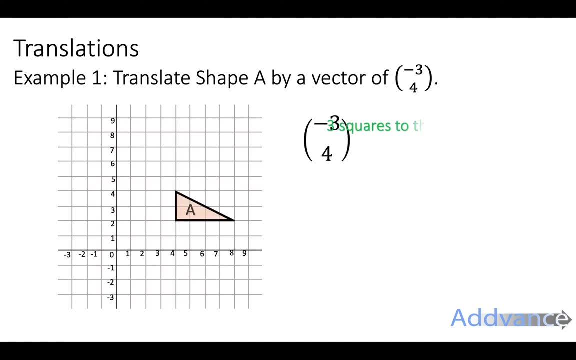 The negative means to the left, the positive means to the right. When it's up and down, the negative means down, the positive means up. So we're going to see an example of this. We're going to translate shape A by vector minus 3, 4.. And so this means minus 3 to the. 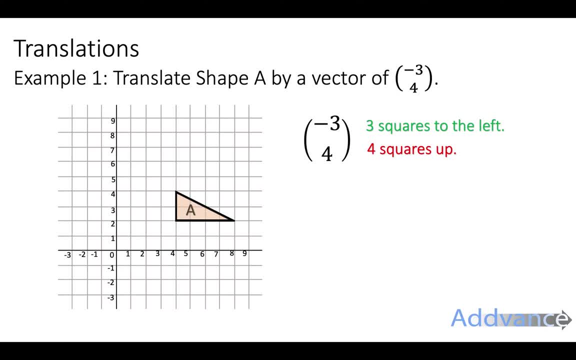 left and 4 squares up. So what we're going to do is we're going to look at each corner individually and we're going to move each corner 3 squares to the left and then 4 squares up. To do this, I like to draw arrows to show what's going on. So the first corner is going to move to this. 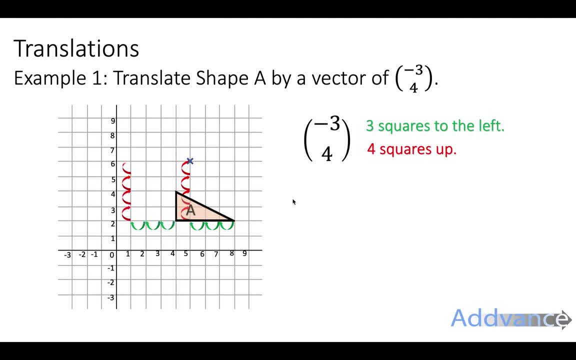 new point, Next corner is going to move to this point And then the final corner is going to move up here. We now know where all 3 corners move to, and we can connect those corners up with a pencil and ruler And we draw it like that. Of course, when we're drawing these, we 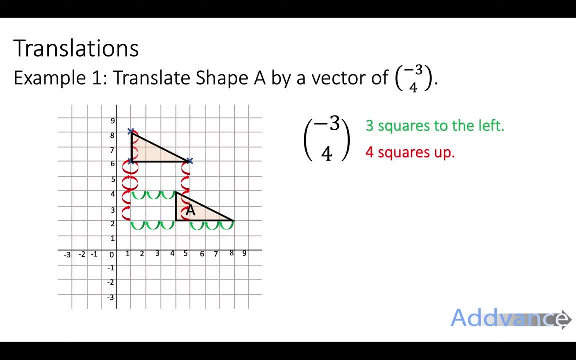 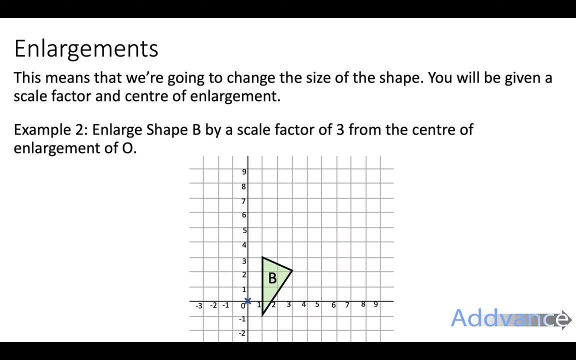 make the diagrams neat with a pencil and ruler, drawn carefully. That's translations. I think it's the easiest one. Now let's talk about enlargements. This means making it bigger or smaller, And you'll be given a scale factor and a centre of enlargement. The scale factor tells you how much bigger 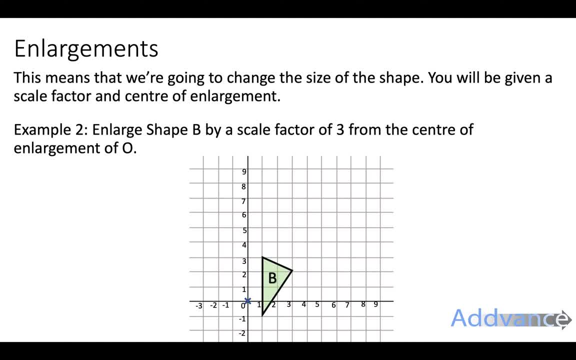 it's going to be and the centre of enlargement tells you where you're going to start when you're making it bigger. So in example 2 we're going to enlarge shape B by a scale factor of 3 from the centre of enlargement O. O means 0, 0. It's short for the origin. So if you see the big letter O, 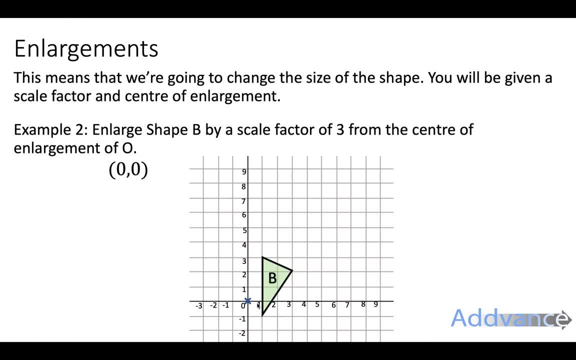 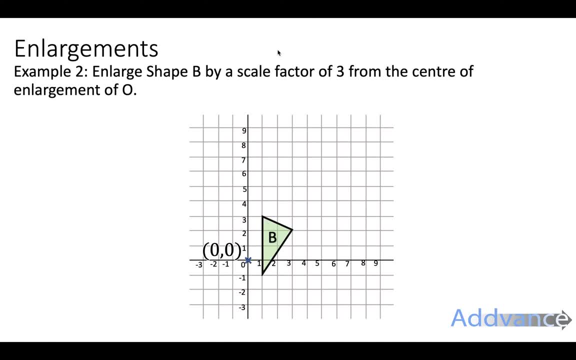 for a corner. it just means 0, 0.. So we're going to start from 0, 0 here and we're going to go through each corner and make each corner 3 times further away, because the scale factor is 3.. 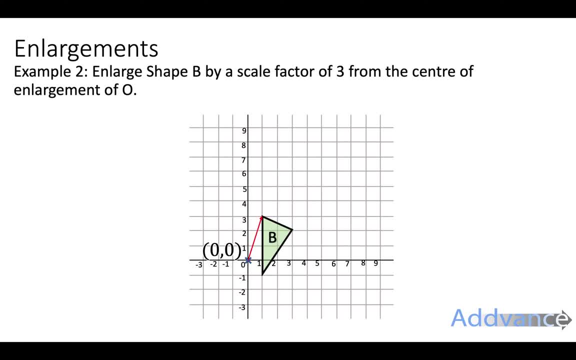 So we get our ruler and we draw a line to the corner and then keep going 3 times further away. Again we do the same and we keep going 3 times further away And for the last corner this is going across 1 square. so we go 1 square, 2 squares and 3 squares 3 times further away. We now know where the 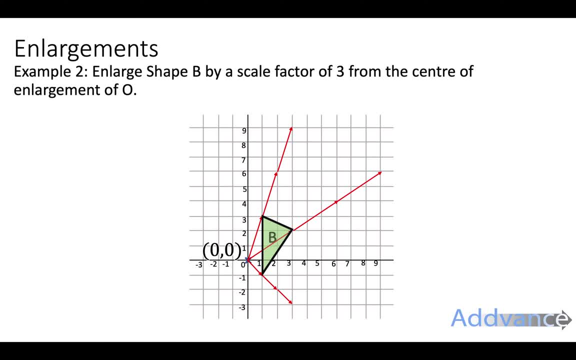 corners will move to and we can connect those up with a pencil and ruler and it will look like this. So we're going to start from the centre of the shape B by scale factor 3 around 0, 0.. In a future video I will talk about negative and fractional scale factors, so please subscribe. 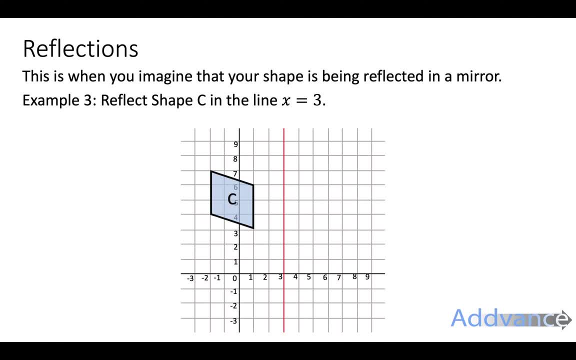 so you don't miss that video Reflections are when you reflect the shape like it's in a mirror, And so this example says: reflect shape C in the line x equals 3.. This red line is the line x equals 3.. So 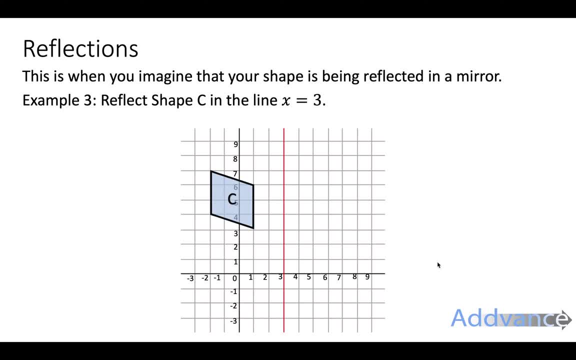 it's 3.. Every x corner on this line is 3, and that's why it's x equals 3.. You will need to remember how to plot straight line graphs for this, so you might want to watch my video on plotting straight line graphs before continuing. 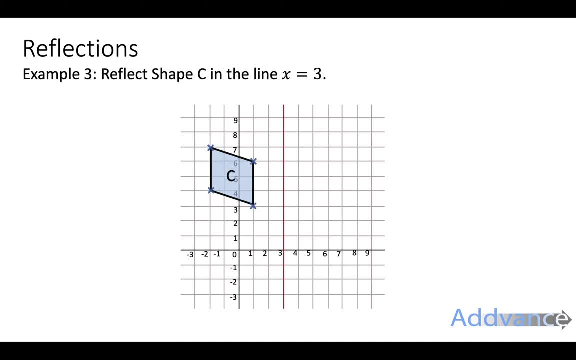 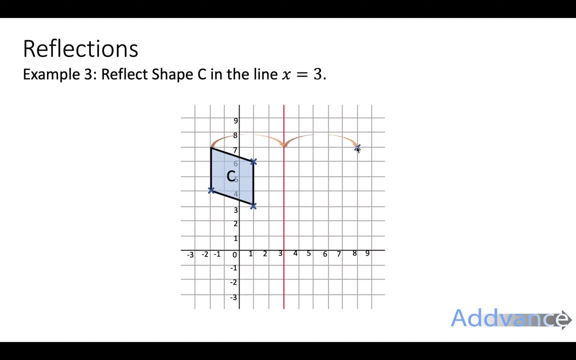 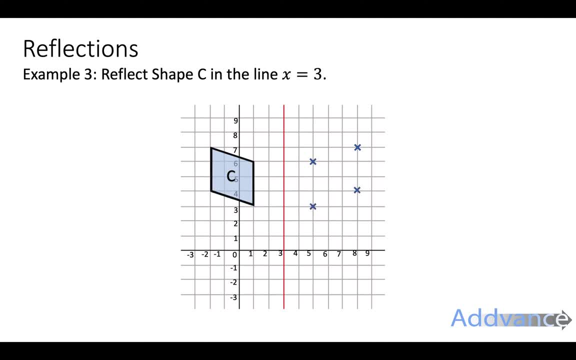 this square and same with this corner. We can then connect them up with a pencil and ruler like this, And that is the final shape. That is the reflection of the shape C in the line x equals 3.. I'm going to show you another example here of 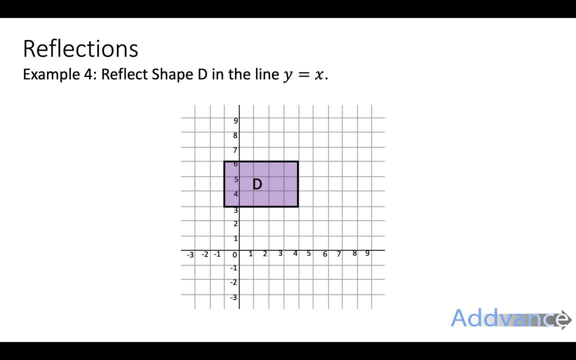 reflection. so we're going to reflect shape D in the line y equals x and we plot the line y equals x to start with like this: Now we're going to reflect each corner individually and this is diagonal. Let's go start with this corner up here and 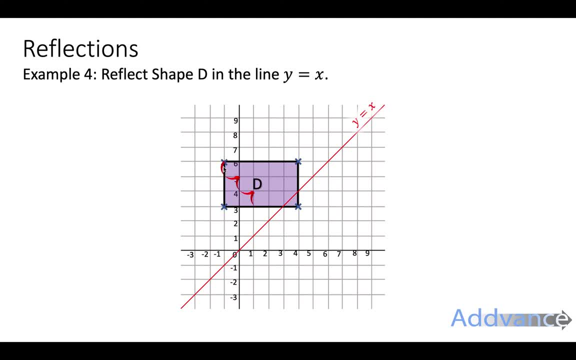 this corner is one, two, three and a half squares from the red line, So we're going to move it another three and a half squares in the other direction from the red line like this, and it reflects to this point over here. Similarly, this square here. 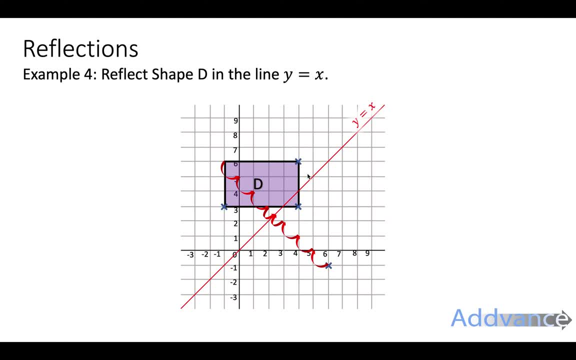 this corner here is going to reflect is one square from the red line, so it's going to end up one square from the line over here like this: This point is on the wrong side of the line, so we move it to the original side of the. 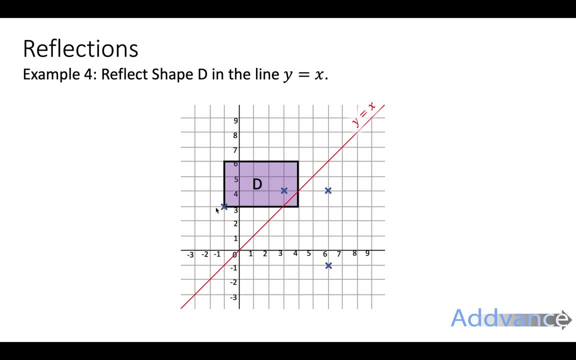 line by reflecting in the line like this, and then this corner will reflect, reflect over here like that. The more practice you get with this, the quicker you'll see straight away where the corners will move to. Then you connect it up with a pencil and ruler and you've done, you've reflected the line. Our final: 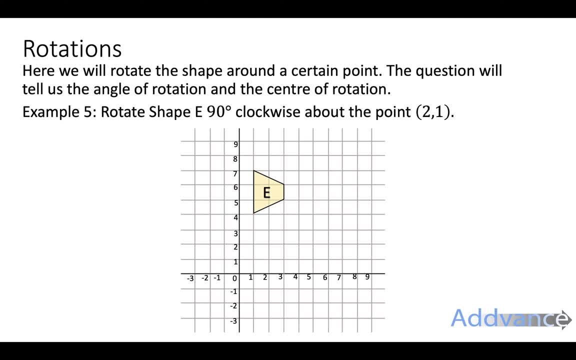 transformation is going to be rotations and here we're going to rotate the shape around a certain point In the question you will be told an angle of rotation and the center of rotation, For example. for example 5, we're going to rotate E. 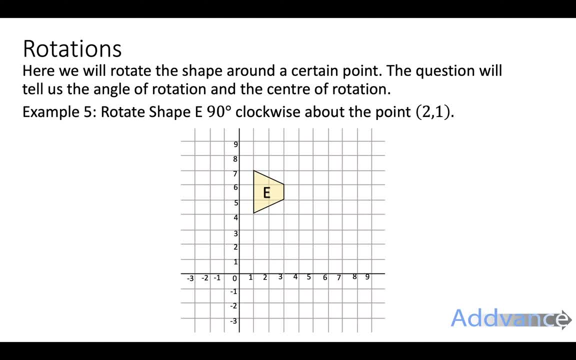 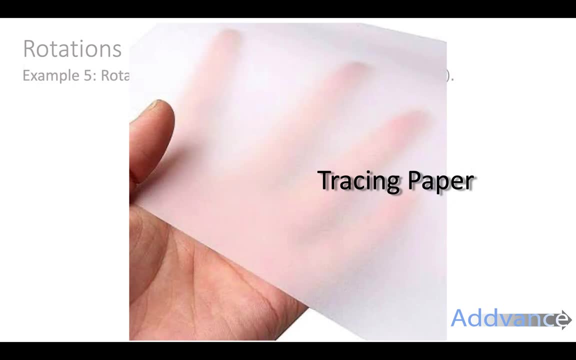 shape E: 90 degrees clockwise, about 0.21.. Remember, clockwise is going to the right and anti-clockwise is going to the left. Just think about how a clock rotates. We're going to need tracing paper for this question. Tracing paper is thin. 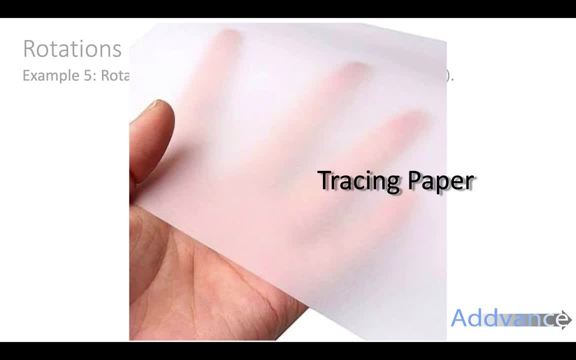 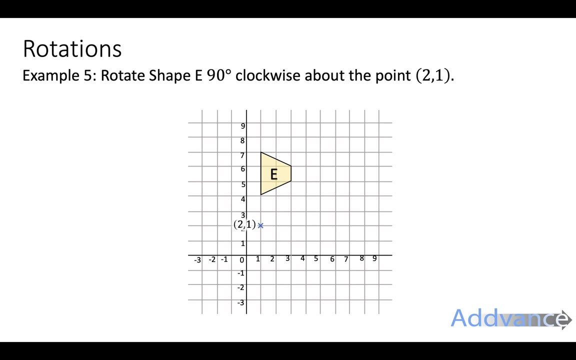 transparent paper that you can draw on. You will be given this in your exam, and so you will need some rotation questions. If you're at home, you may use baking paper. We mark on the corner 2: 1 here, and then we take our. 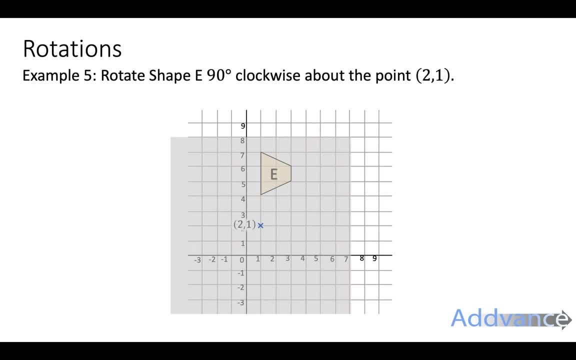 tracing paper and we place it over the top. Then on tracing paper we mark the corners of the shape like this: with our pencil. We draw them with a pencil on the tracing paper over the top. We then take our pencil and we rotate it around the point 2: 1. Use your pencil as an anchor If you press hard on the